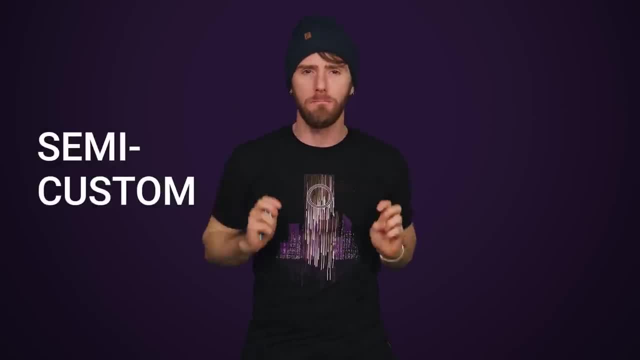 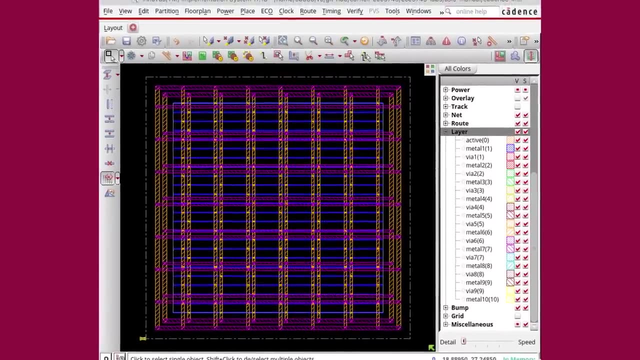 Some ASICs are manufactured in what's called a semi-custom manner, where the fab has what's essentially a blank template of logic gates which are then permanently connected according to the design the client needs. Meanwhile, other ASICs are full custom designs. 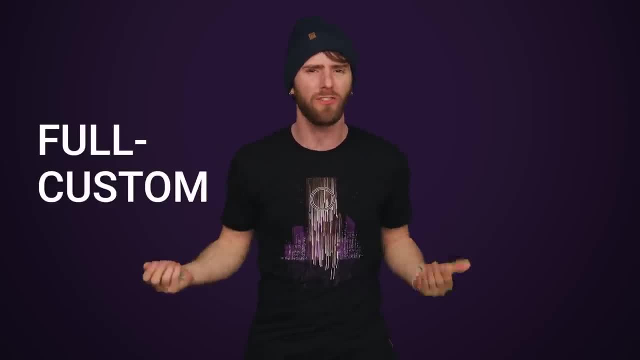 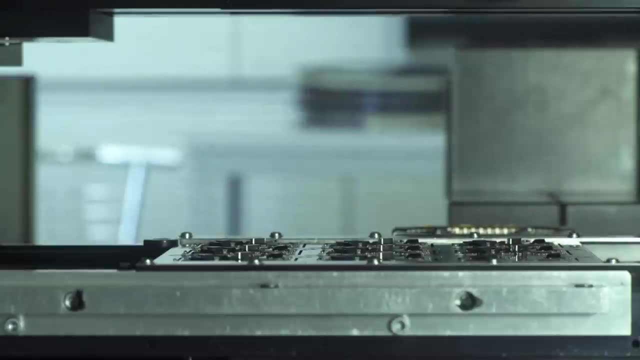 where the entire chip and every transistor is pretty much designed from scratch. Unsurprisingly, because ASICs are so specialized, they take a lot of time and money to develop, But because ASICs are usually for small, highly integrated devices that ship lots of units, 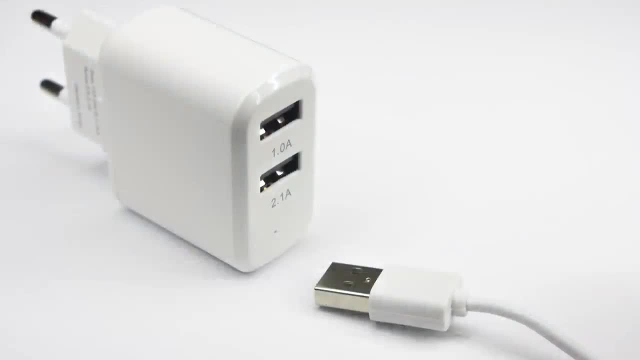 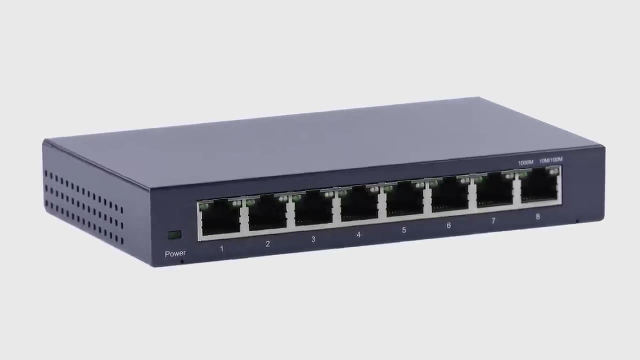 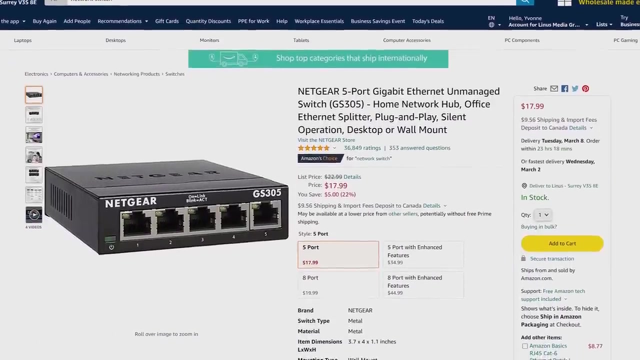 the cost of an individual ASIC tends to be quite low. For example, the chips inside USB chargers or network switches or even electronic toys are often ASICs, but all of these are often low cost products. Network switches are a particularly interesting application, since a simple $15 unmasked ASIC 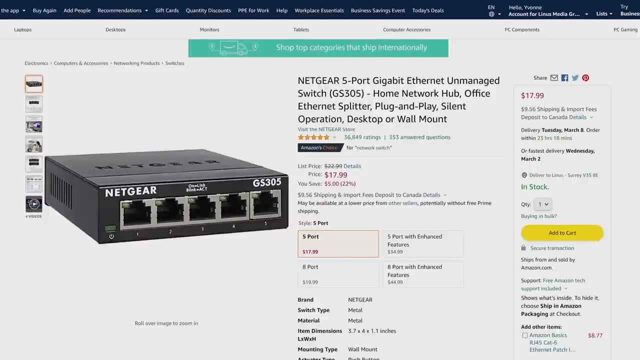 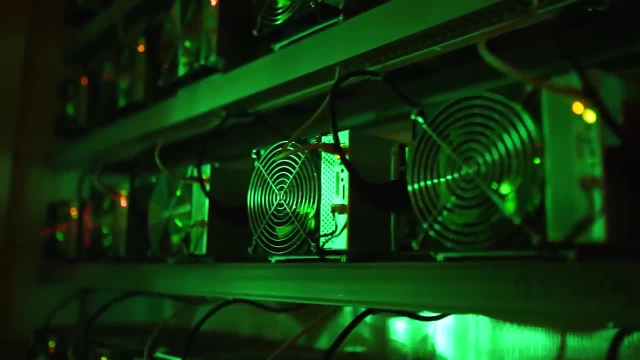 or $20 unmanaged switch can handle network traffic better than a desktop CPU that costs 10 times as much. But of course there's a good chance. you've heard of ASIC-based crypto miners designed to run cryptographic hashes much more efficiently than a graphics card can. 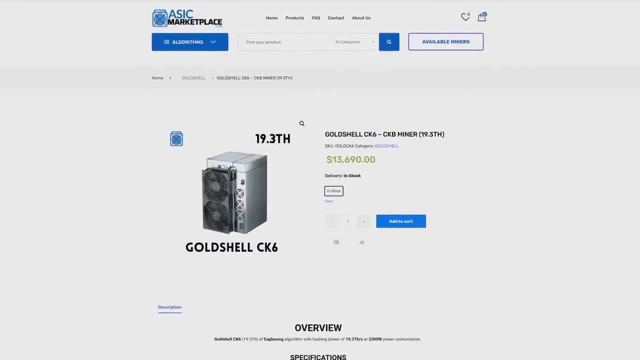 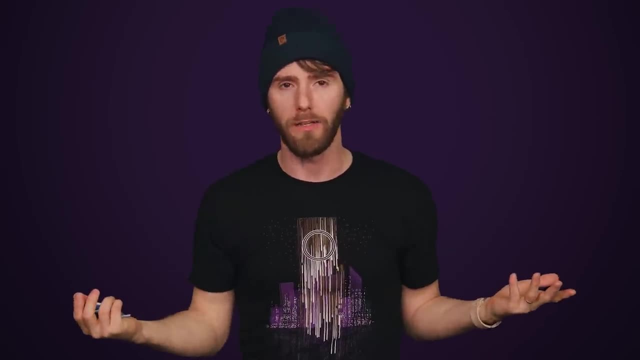 And those are quite expensive due to both demand and the fact that they aren't as mass produced as other ASIC-based devices. And of course, there's the fact that they make you money. We'll tell you about the other kind of chip we're discussing today, the FPGA. 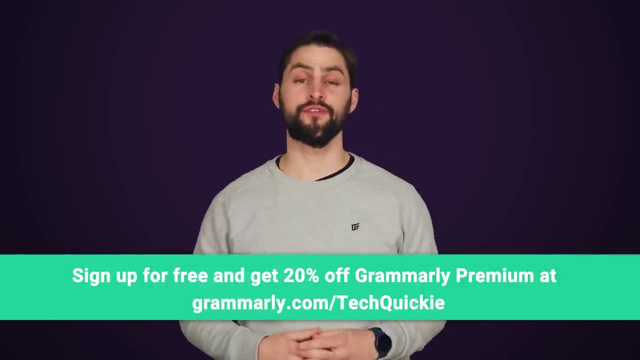 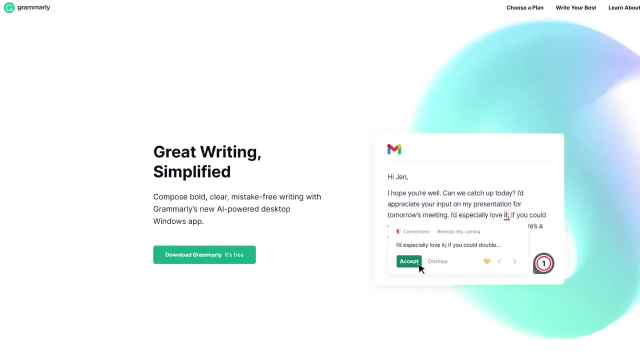 right after we thank Grammarly for sponsoring this video. Thanks to Grammarly for sponsoring this video. Communications through online email, Slack or Discord can be easily misinterpreted and it can become a huge time block. This is why all working professionals need a tool like Grammarly. 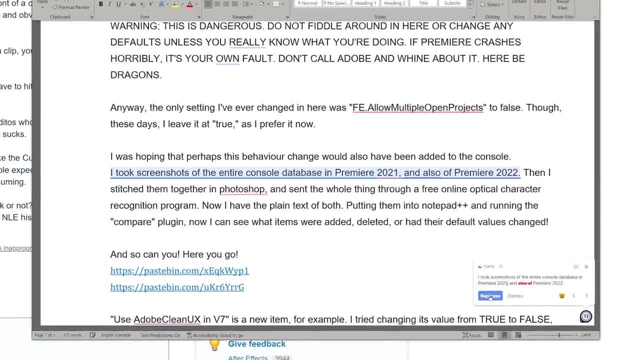 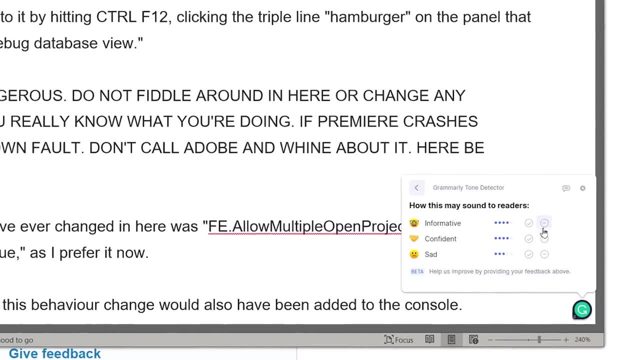 There's also Grammarly Premium, which provides more in-depth feedback on your writing so you can really learn. We recommend checking out the tone transformation and clarity tools. Oh boy, I could use that. I'm a jerk. They help you by rewording phrases. 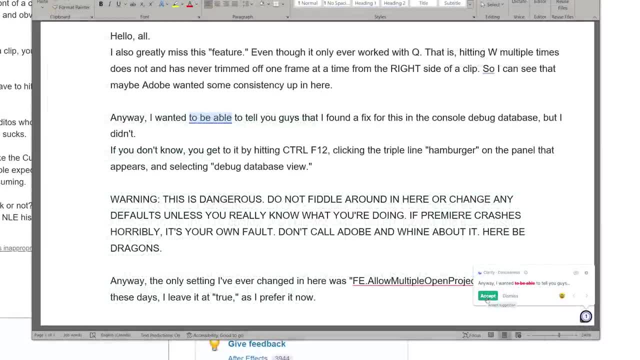 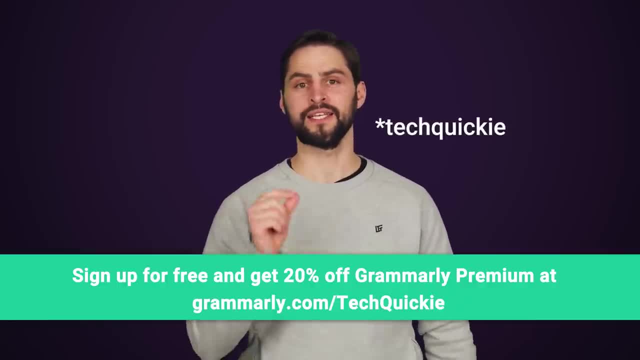 to make you sound more confident and by removing unnecessary jargon, to help you get your point across clearer, more clearly. Work smarter, not harder. Go to grammarlycom slash techlinked to sign up for a free account and get 20% off Grammarly Premium today.